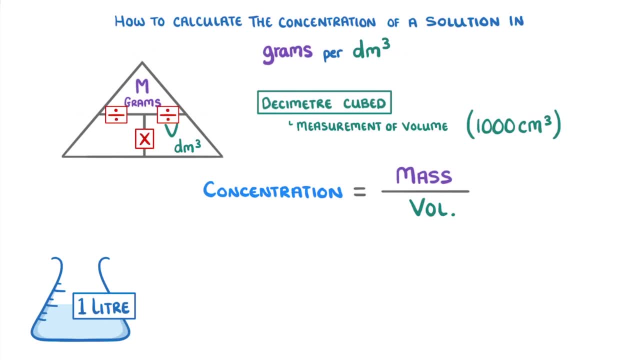 find the concentration, we'd cover up the C and do mass divided by volume. Or if we wanted the mass, we'd do concentration times volume. Finally, if we wanted volume, we'd do mass divided by concentration. So if we had 40 grams of sodium hydroxide dissolved, 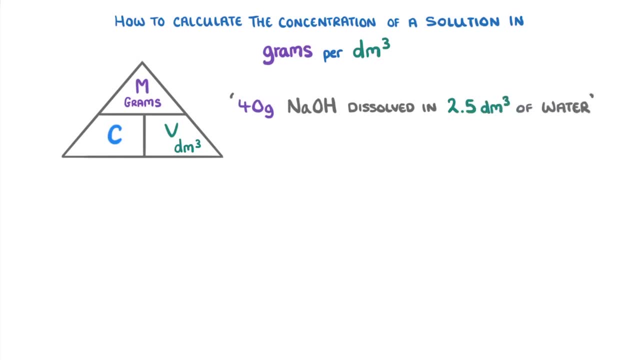 in 2.5 decimetres cubed of water, the concentration would be 40 grams divided by 2.5 decimetres cubed, so 16 grams per decimetre cubed, And instead of writing per decimetres. 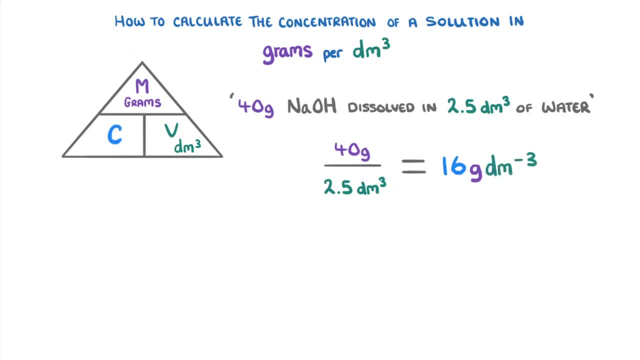 cubed. every time we can just write dm to the power of minus 3, as the minus here means the same thing as per. Or, if we had 24 grams of copper sulphate in 480 centimetres cubed of water, we would first divide the 480 centimetres cubed by 1000, so convert it to 0.48 decimetres. 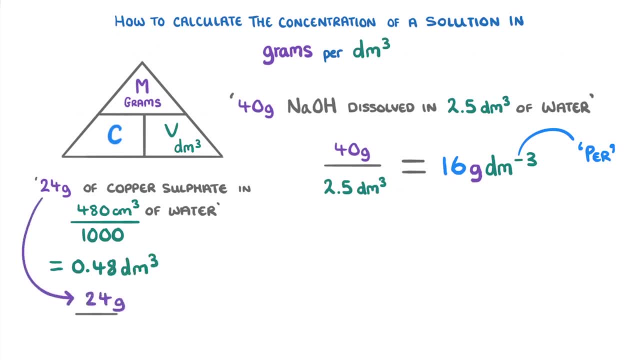 cubed and would then do 24 grams divided by 0.48 decimetres cubed to give us our concentration of 50 grams per decimetre cubed. As you can see, in this question it's always important to check the units of the figures you're given, as being given things in kilos instead of 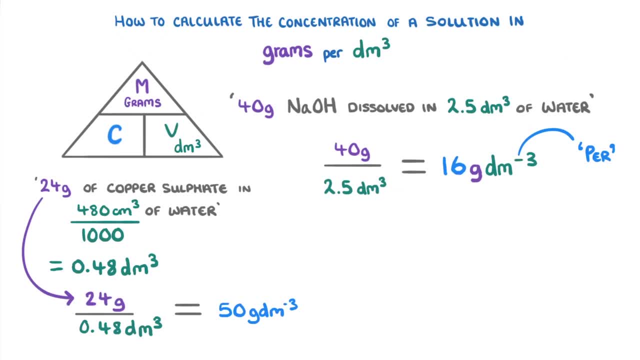 grams or centimetres instead of grams, is a very important thing to do, So let's start with the units of the figures you're given, and then we'll look at the units of the figures you're given Now. we said at the beginning that we can also use this equation to work out the mass, if. 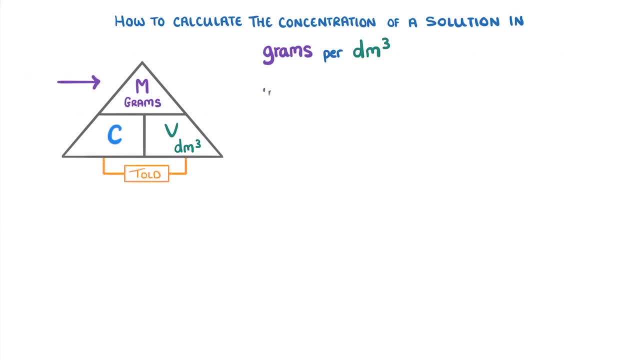 we're told the concentration and volume. For example, a 400 centimetres cubed sample of hydrochloric acid has a concentration of 20 grams per decimetre cubed. What mass of hydrogen chloride is in this solution? If we look at our formula triangle, we can see: 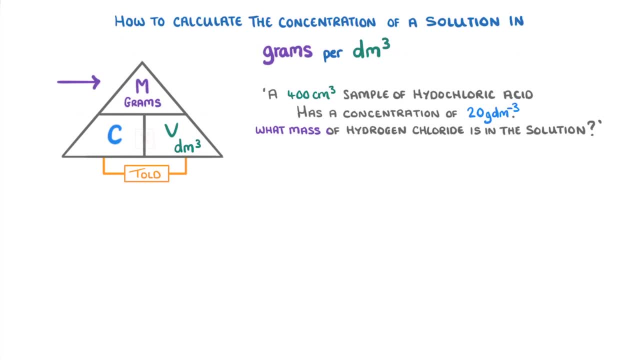 that the mass of hydrogen chloride which is on the top must be concentration times volume. So we just turn our 400 centimetres cubed into decimetres cubed by dividing it by 1000, and multiply this 0.4 decimetres cubed by 20, to give us a mass of 8 grams. So there,